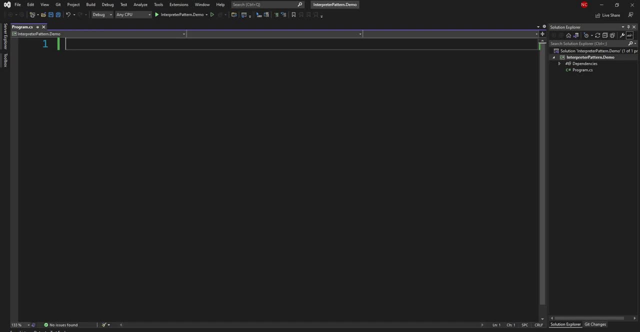 Now, when it comes to interpreter design pattern, there are three main players in this design pattern. The first one is the context. The context will contain both the value, which is a string in most cases, especially when we are dealing with a command line argument, and an expression which is 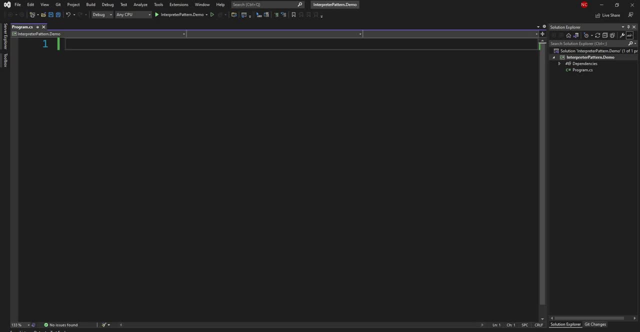 some sort of character using which will understand what action to take, and then it will have an expression evaluator which evaluates the expression to understand what to do. and then, finally, we will have an interpreter which takes the incoming string and the expression and then works with the expression evaluator to ultimately interpret the expression and provide the output. 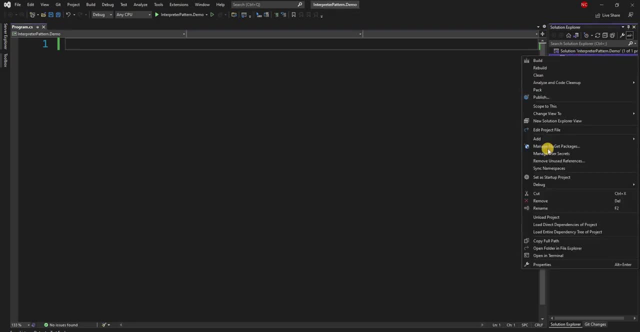 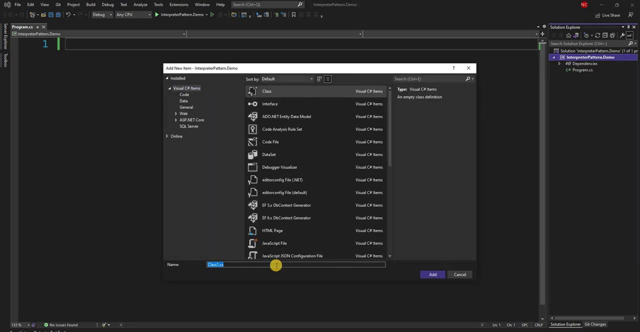 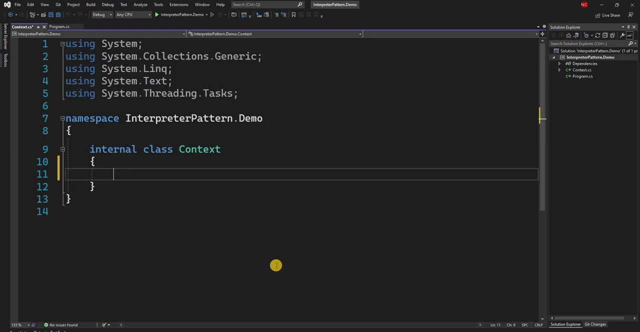 So to do that, first we are going to create a context class, which is going to be a simple class, which will have two properties: a value and an expression, and in our case, both will be string. So we are going to create a context class and we can create a constructor. 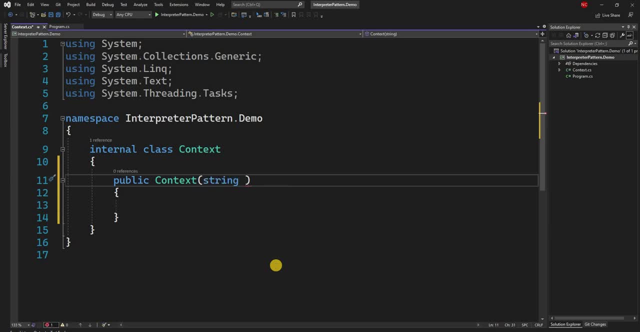 and here we'll have string expression and string value and we can create both as properties. The value will provide as a setter also, because it will be manipulated from the interpreter. and then next, what we are going to do is we are going to create the expression. 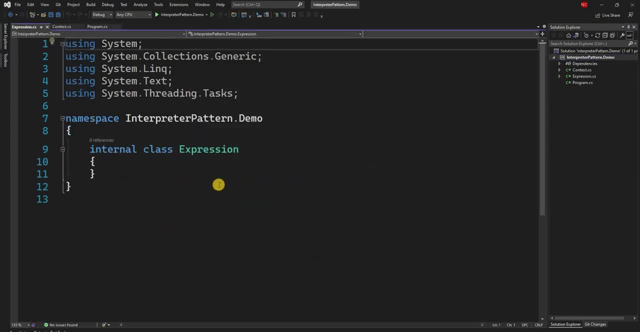 Now for our example. what we want to do is that we want to handle a command line argument to convert a string into lower or uppercase. So what we're going to have is we're going to first have an argument and then we're going to create a setter, and then we're going to create an expression. 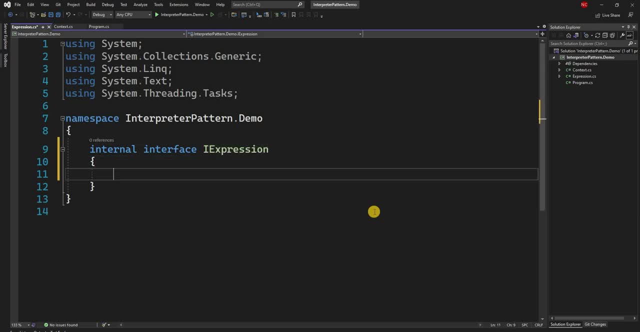 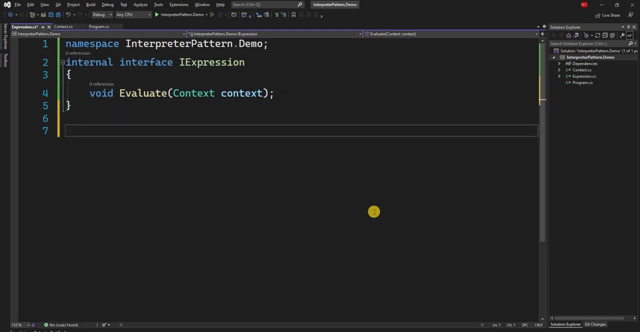 So what we're going to do is we're going to create an i expression, which is an interface, which will have a single method called evaluate, and it will take the context, because it is going to work on the context for evaluation and for us, we're going to have two types of expressions: a lowercase expression and an uppercase. 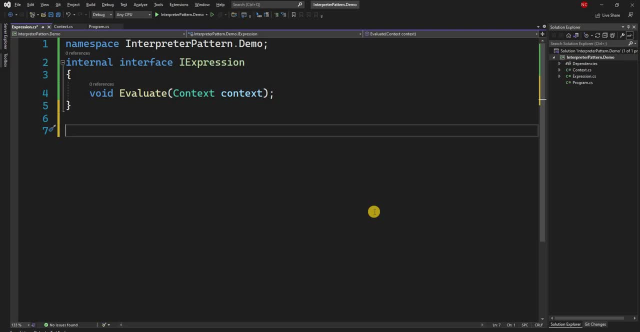 expression, because that's all we are going to handle, at least for this example. So we're going to create an internal class, lowercase expression, and here all we are going to do is we're going to say context dot value is equal to context dot value, dot two lower. 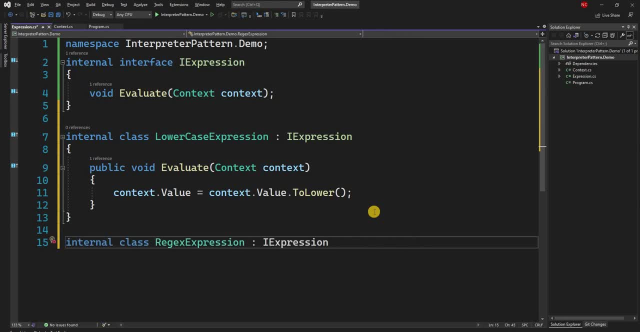 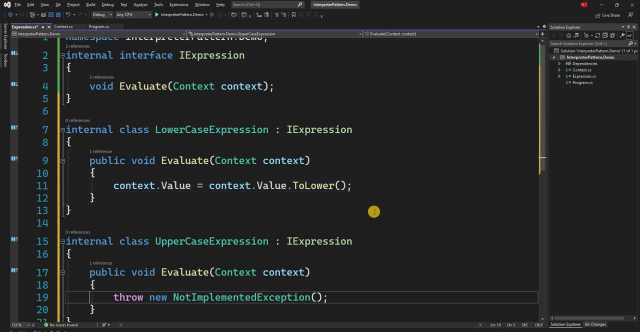 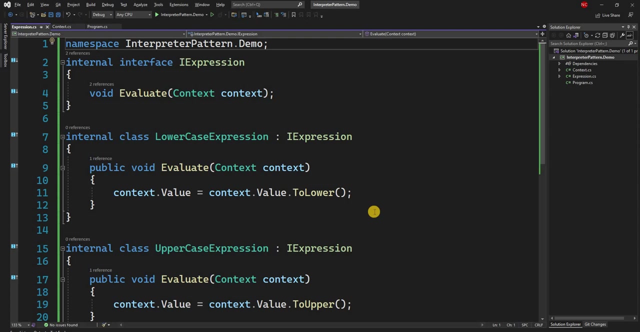 And similarly, we're going to have another class called uppercase expression and here, similarly, we're going to have the context value is going to change to two: upper. These are the two expressions that we are going to have, And now we define the context, we define the expressions. 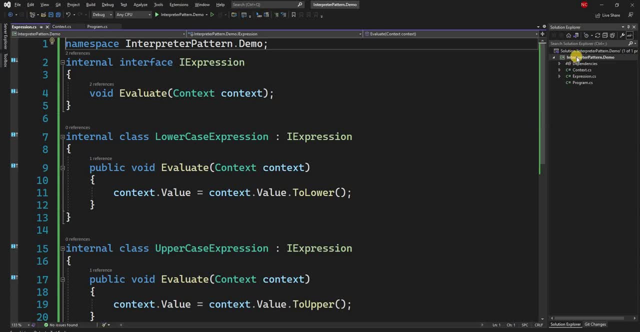 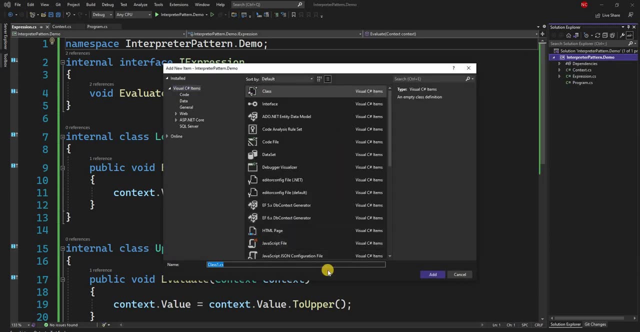 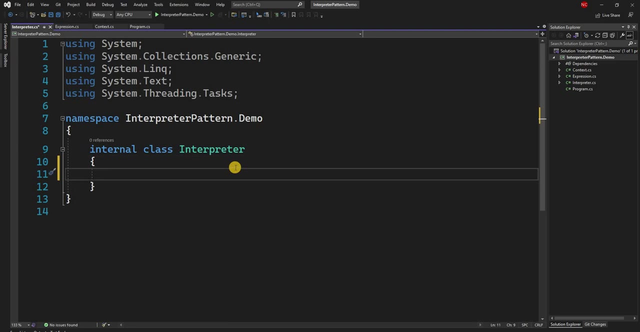 We are going to support two expressions. Now it is time to create the interpreter, which is going to ultimately use the expression to interpret the incoming message. So for the interpreter class we are going to have a single method. so public void interpret, and interpret is going to take a context. 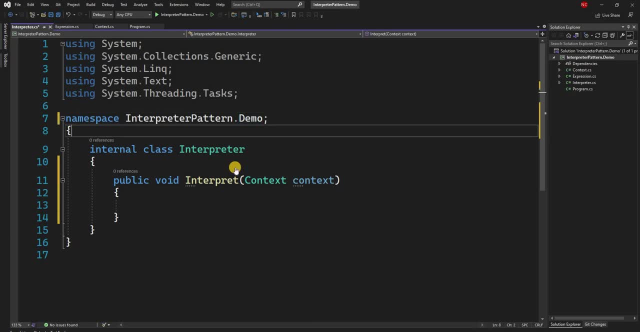 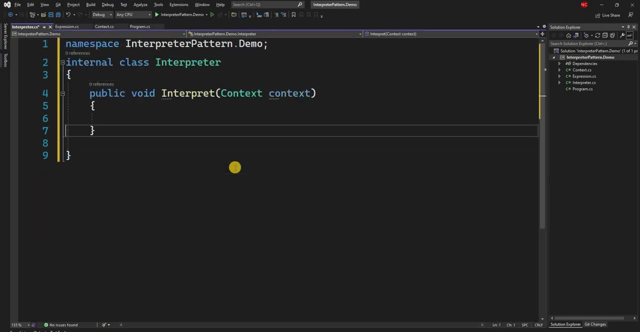 So we are going to have a single method, so public void- interpret and interpret. So we are going to have a single method, so public void- interpret and interpret. And next, what we're going to have is here: first, we are going to get the expressions. Now, remember, the expression can be a set of. 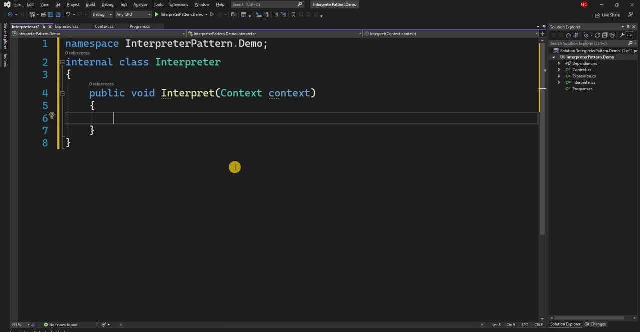 expressions. In our case, or in this example, it does not make sense to have a set of expression, but there are cases where you will have set of expressions. So we are going to support a set of expressions. So it will be var equal to. and here we are going to split based on space. That's our splitting criteria. 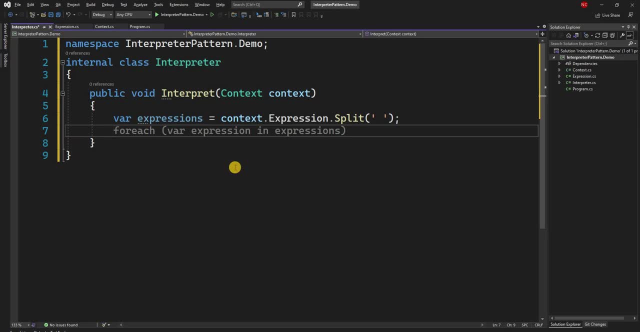 And then what we can do is we can create the types of expressions. This is basically going to be our syntax, which we are finding out later in the show on school. We're not necessarily going to " going to be a new list of i expression, because at this point we will be. 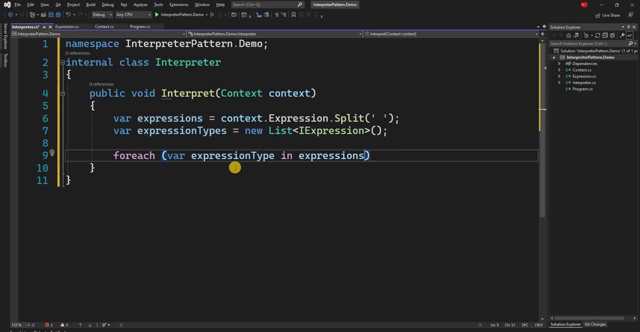 creating the expression. and then what we can do is we can create for each loop of expression, and here we can say: if expression expression is equal to dash L, then we want to add the lower case, lower case expression into our expression types area and LC if expression is equal to dash you. what we are going to do is we can now say: 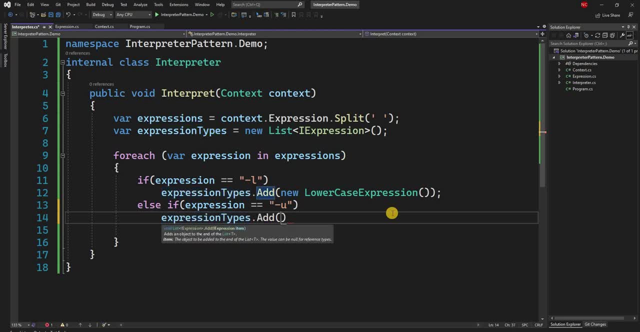 expression types: dot add. and here we are going to say new upper case expression and then after that, what we are going to do is, now that we have identified which expression is going to use which expression type, that means we have done half of our interpretation. now it is time for us to evaluate the 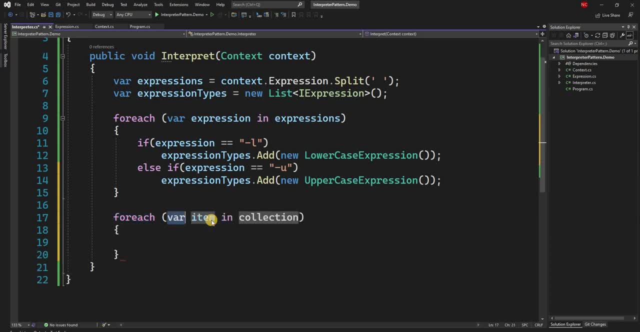 expressions. So then what we can do is we can have another for each loop and we can say item in expression types. and then what we are going to do here? here we are going to say item dot evaluate, and we are going to pass the incoming context and after everything is evaluated we can just use console dot. 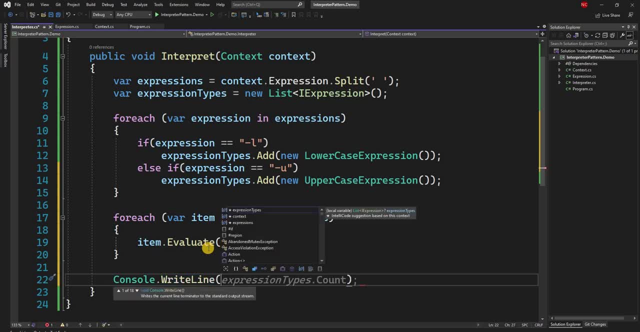 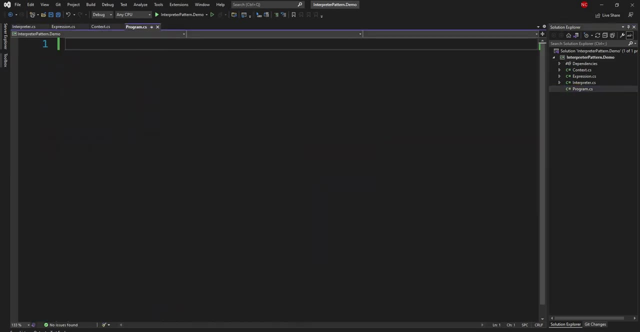 right line. and here we can do the context dot value, because the value would have been mutated, based on the expression, into the desired outcome. as simple as that. and then what we can do now is we can go into the program and in program, what we are going to do is we're going to say: 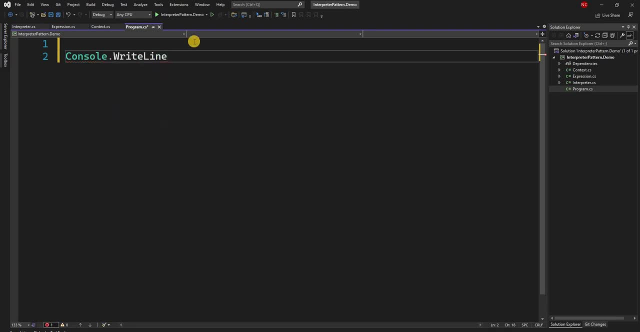 console dot right line, because this is where we want to get the input from the user and we can say: provide a word with expression and then we can say var word is equal to console dot read line and then what we can do is we can extract the value out of it. 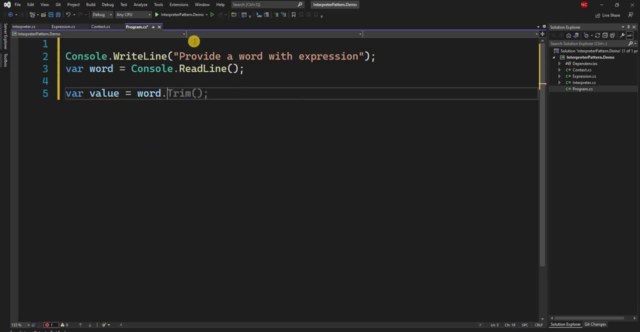 so we can say: value is equal to word dot. substring of 0 and the length is word dot. index of dash: anything before dash is what is our word. and then for the expressions, what we can do is we can say bar expressions and here we're going to say expressions is equal to, again, word dot substring. 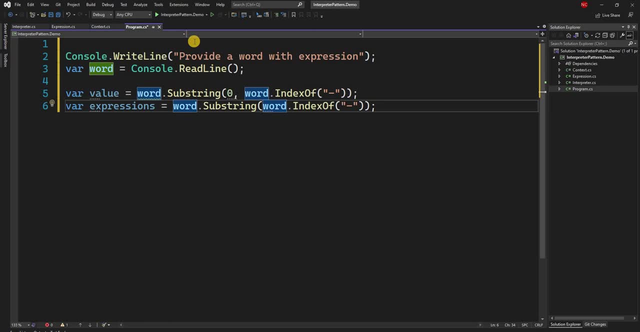 but here the index, where it starts from, is the index of dash and till the end of the user's input. and next what we are going to do is we're going to create interpreter. it's equal to new interpreter and here interpreter does not have any constructor and i have to add the namespace and then what we can. 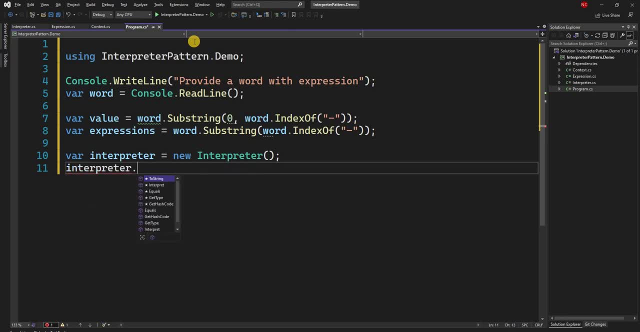 do is we can do interpreter, dot interpret, and for the interpreter it takes a context, so we can create a new context and the first parameter is the expression and the second parameter is the value. so now, if we run this, so now if we run this application and if we pass a word or a sentence- actually it should have been provide a sentence- 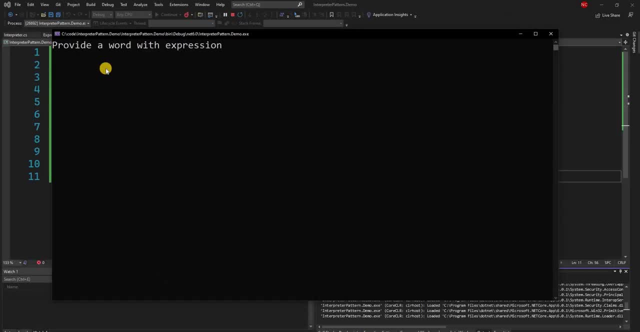 because i'm going to provide a sentence, not a word, but that's okay. so if we say hello there and if we pass l for lowercase now, it converted the entire sentence into lowercase. similarly, if we pass and you pass lowercase, lower and then upper, now here, what is going to happen is it is going to add both the expression. 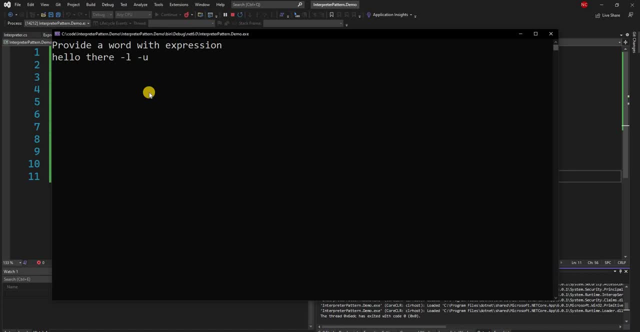 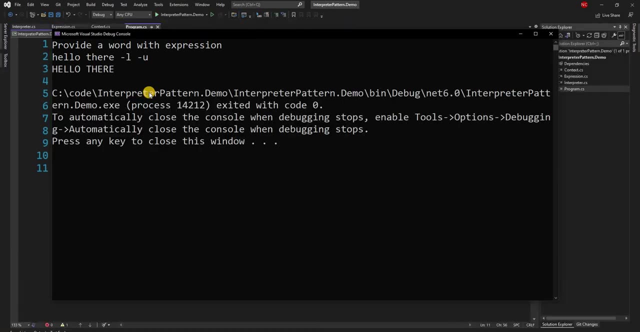 lower as well as upper, but since it is adding lower fast and upper later, upper will be executed second and it is going to convert everything into uppercase and as expected. and from here you can see that we can create for a particular input, we can create multiple expressions and we can do.